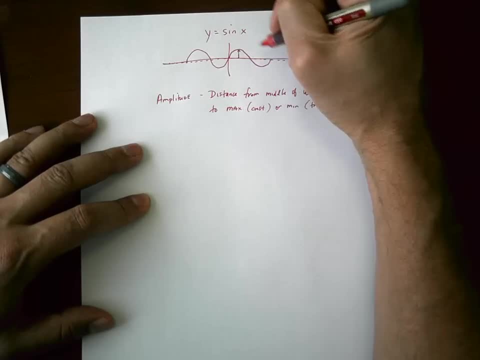 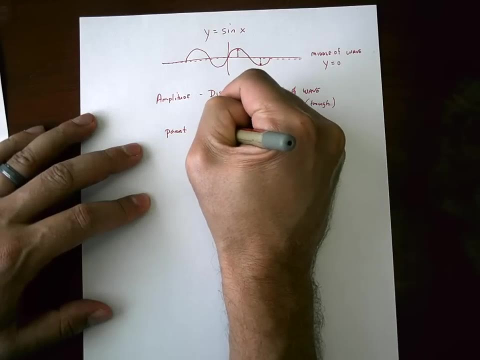 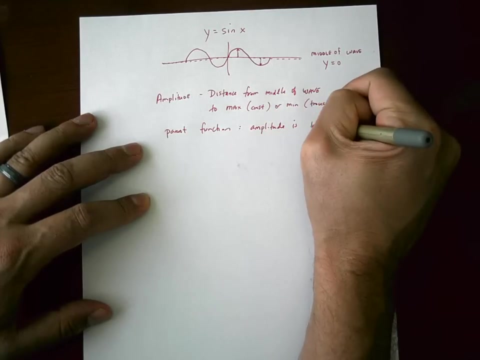 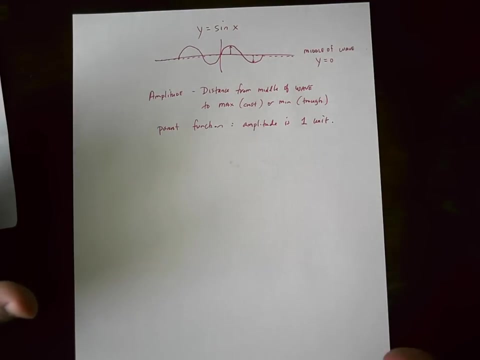 So the amplitude is the distance from the middle of that wave to the maximum or the minimum. So, on the parent function, the amplitude is one unit. So our concept we've been talking about is a vertical stretch or a vertical shrink. Well, when you do a vertical stretch, 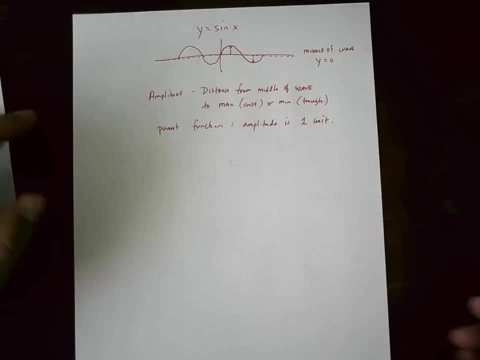 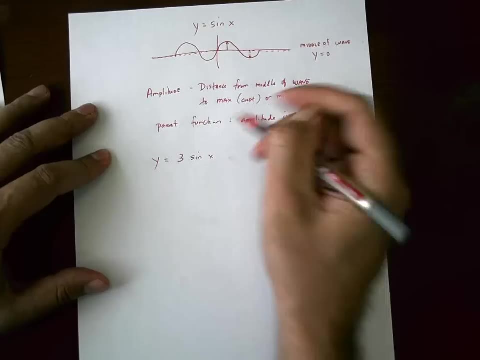 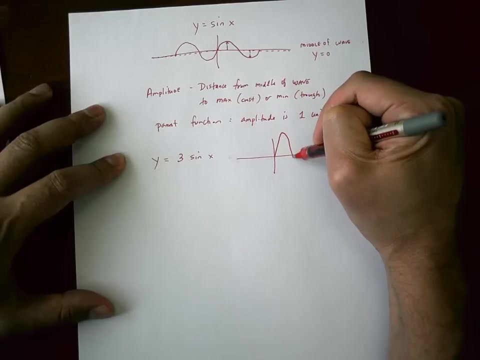 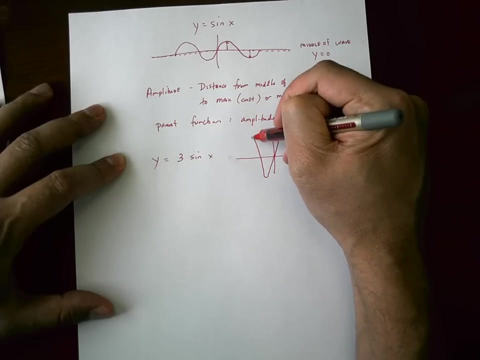 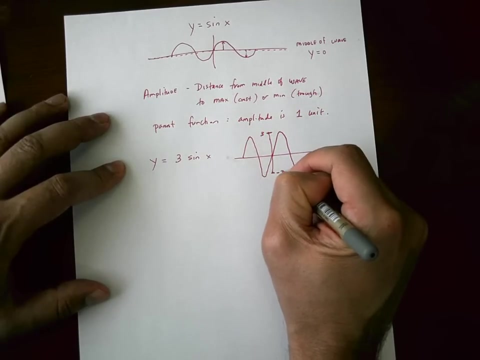 stretch or a vertical shrink. you're just. you're just changing the amplitude. so if the function is y equals 3 times the sine of X. right, the transformation that occurs is you have the same x-intercepts, but now your output is hitting a maximum up here at 3, and it's hitting minimums- bad drawing there- at negative. 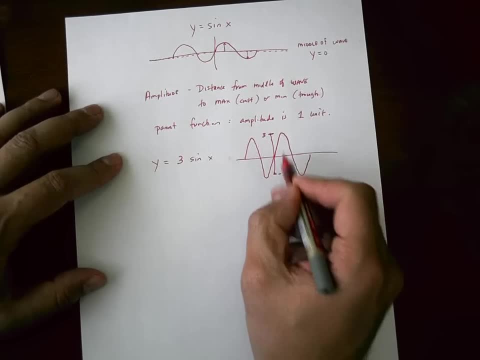 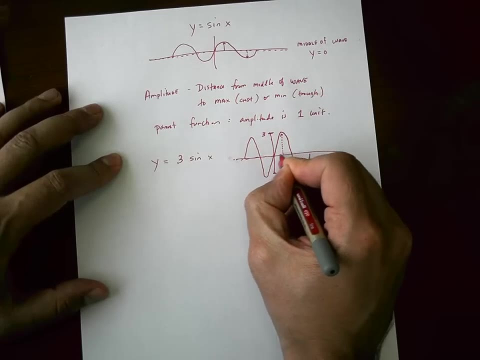 3. right, so the amplitude? you'd say, oh, that's a vertical stretch by a factor of 3. well, you're also changing the amplitude. this distance from the middle of the wave- the middle of the wave is still at- y- equals 0. you still have the same x-intercepts. this is at 180 degrees. this is at. 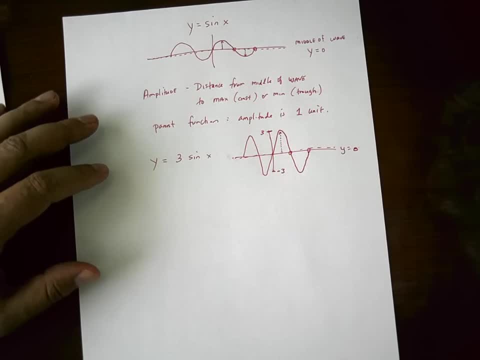 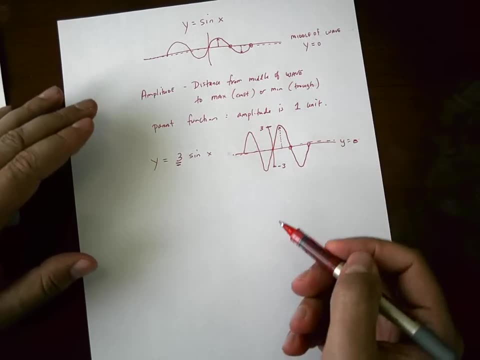 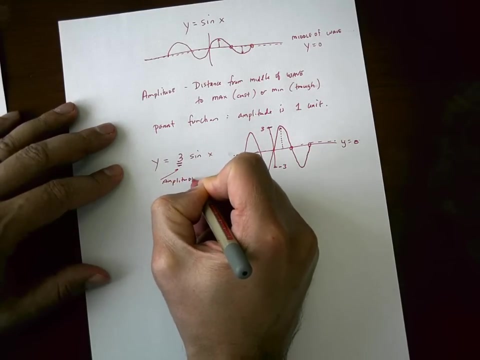 180, this is at 360, this is at 360, or pi, 2pi, but you change your amplitude. so this value right here that's causing a vertical stretch or a vertical shrink, that value is the amplitude. now students sometimes get confused, put a negative sign like, say oh, what if it's negative? 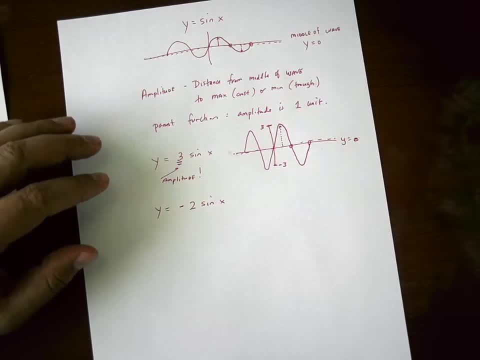 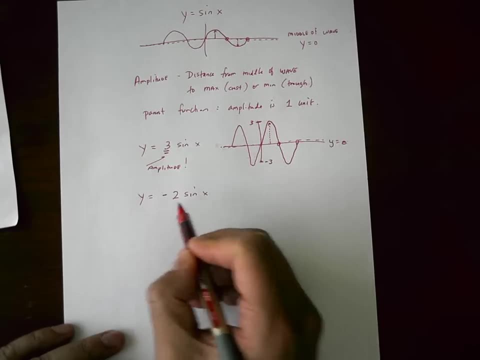 2 times the sine of X and you say: what's the amplitude of that function? let's say the amplitude. Oh, you told me it was this value in front of here. so the amplitude is negative 2.. No, the amplitude is not negative 2.. 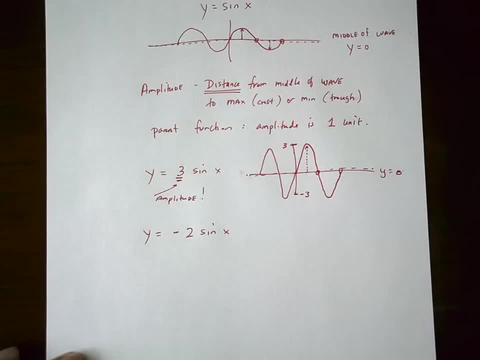 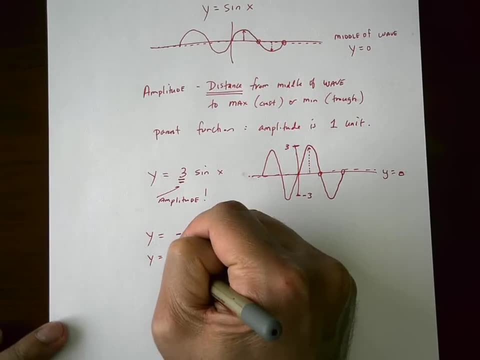 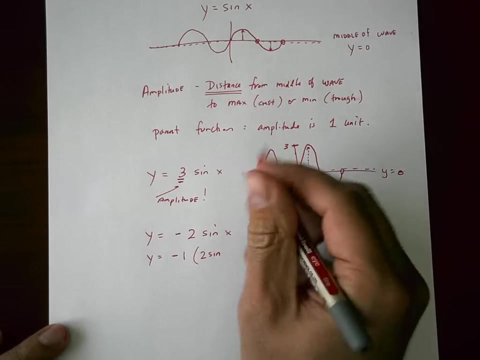 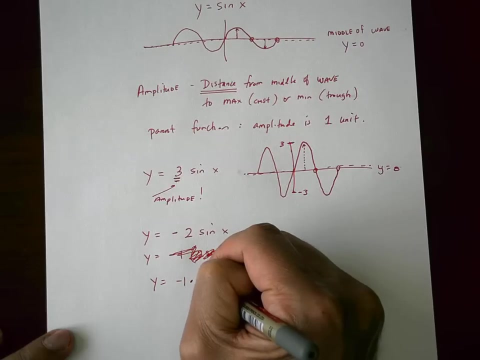 Amplitude is a distance and distance is not negative. When you see that negative 2, you've got to think of it as y equals, in essence, negative 1 multiplied by. I don't even want to go that route. You've got to think of it as negative 1 multiplied. 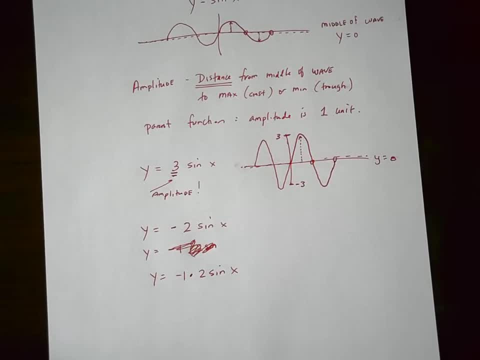 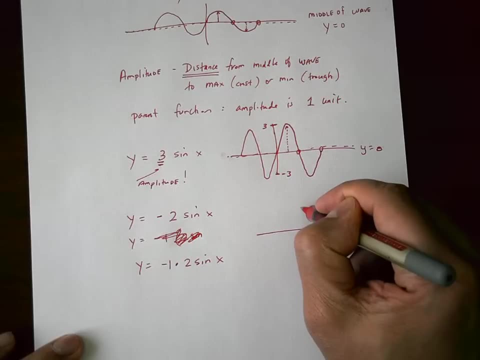 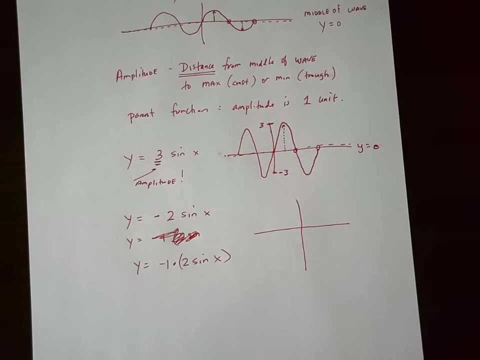 by 2 times the sine of x. That's what negative 2 times the sine of x means. And so, graphically, remember multiplying the output that has been produced from 2 times the sine of x. it's then multiplied by negative 1.. 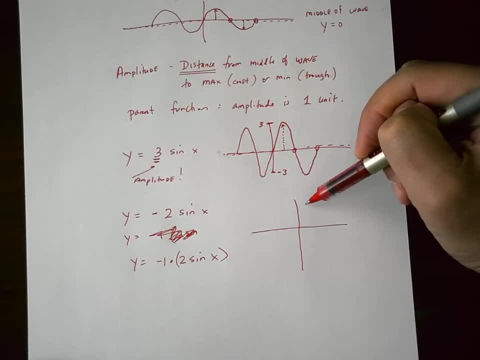 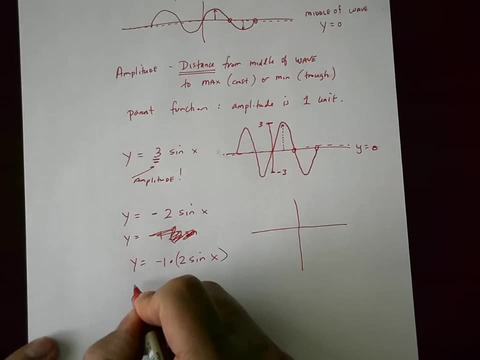 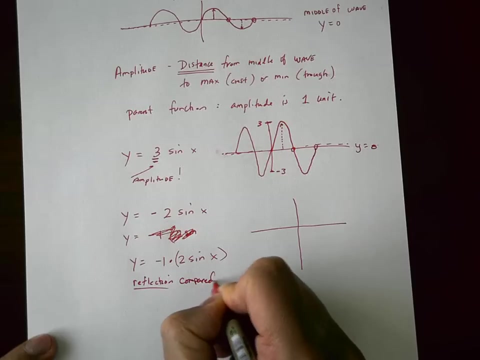 And so you get a switch of your output values. All your output that used to be positive is now negative, and all of your output that used to be negative is now positive. That's a reflection. That negative sign causes a reflection compared to the x-axis. 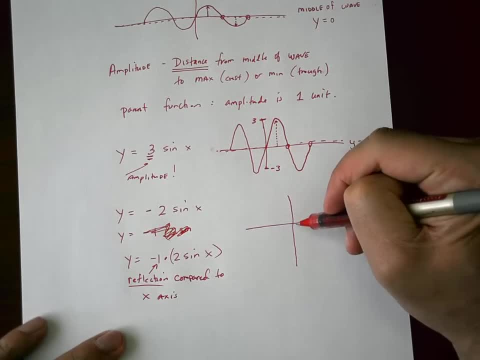 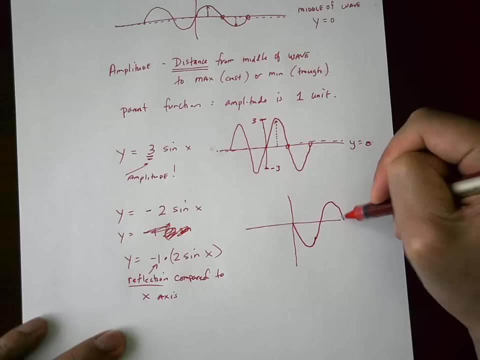 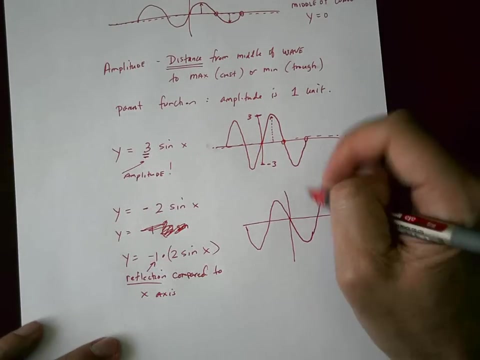 So 2 times the sine of x, instead of going up here to positive 2, you're going to get a reflection. It's going to be something like this, And so you'd say: what's the amplitude? Well, the amplitude is still positive 2.. 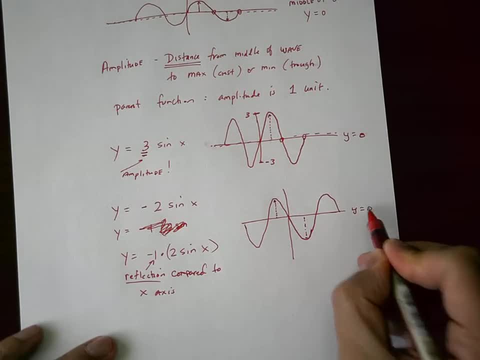 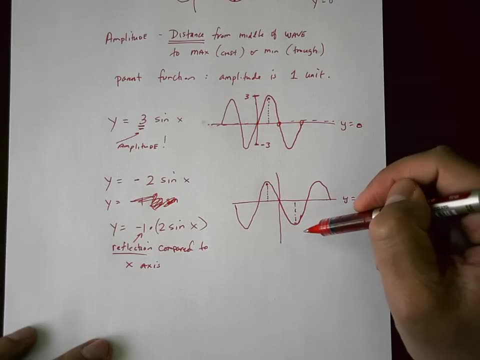 The distance from the middle of the wave- the middle of the wave is still at y- equals 0. The distance from the middle of the wave to the maximum, or the minimum, is still 2 units. So if the function says, y equals negative 2 times the sine of x. 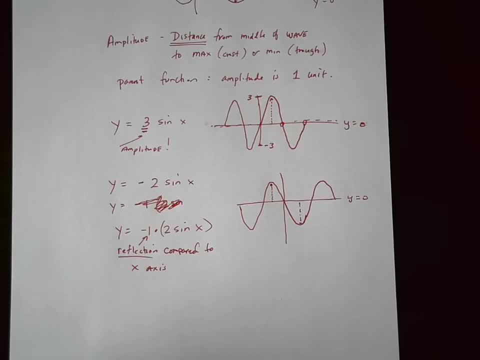 say: What's the amplitude? The amplitude is 2.. It's not negative 2.. What about the negative sign? Well, it's changing all of the output values from positive to negative, negative to positive. It's causing a reflection compared to the x-axis. 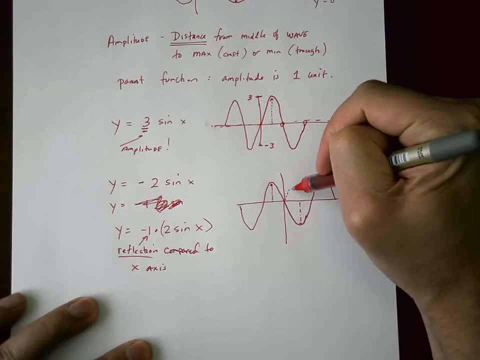 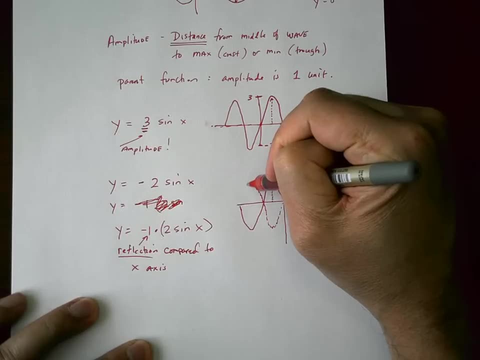 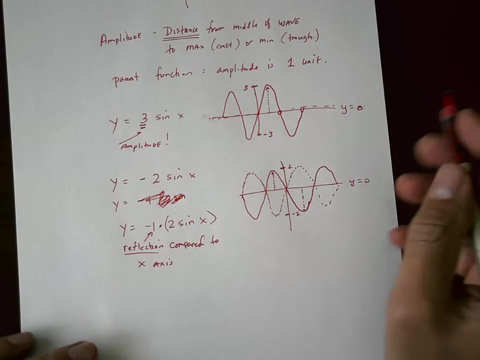 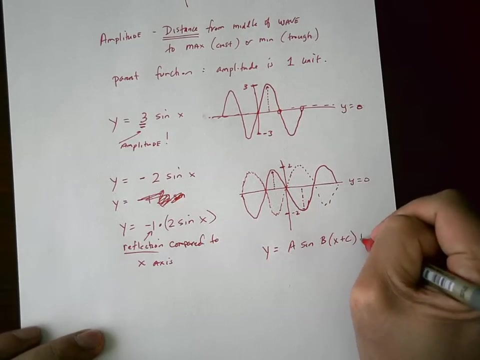 If the negative sign wasn't there, it'd be like this: This being up here at 2, and this being at negative 2.. What's the amplitude? So when we're writing functions and we say y equals a times the sine of b multiplied by x plus c plus d. 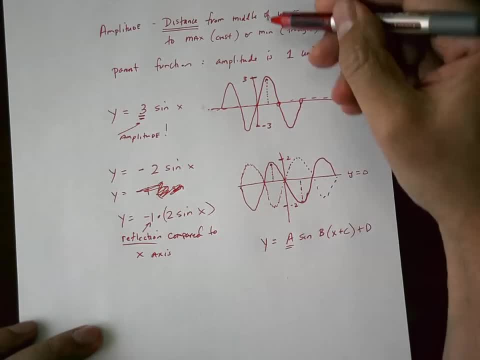 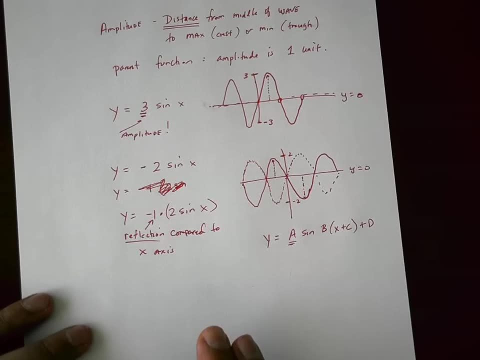 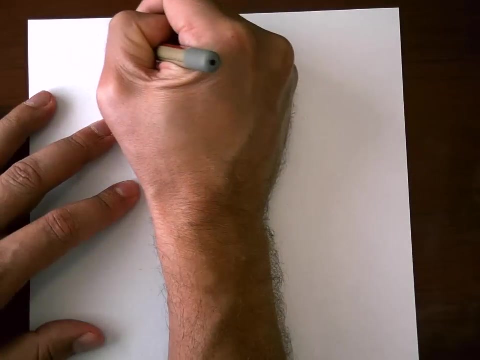 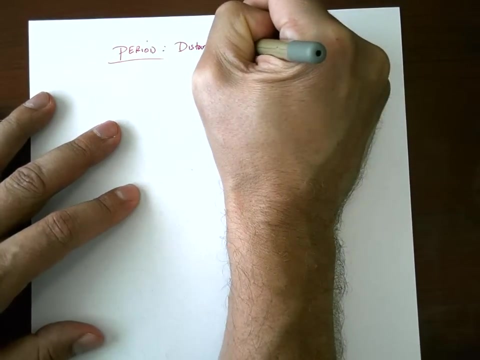 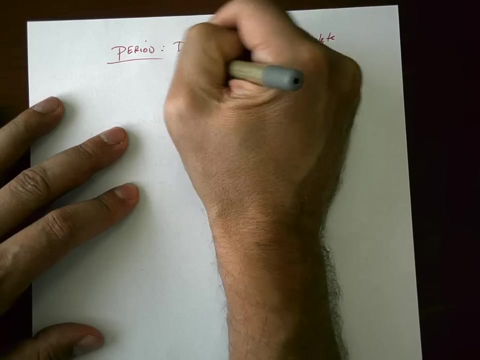 this value here. that affects vertical stretch or vertical compression. that is your amplitude. Now we need to talk about the concept of period. OK, Period Period is technically the distance, or in our applications, it'll be the time to complete one cycle. 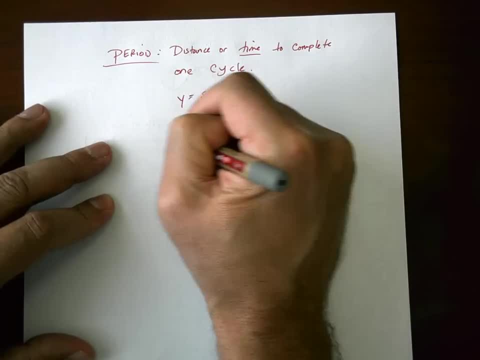 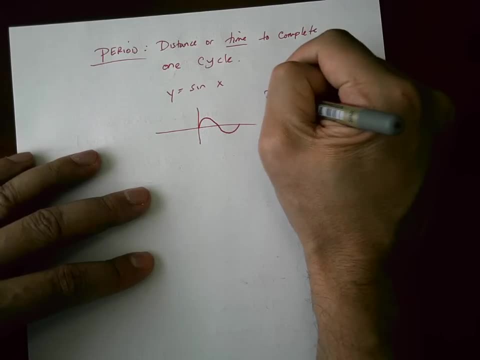 And so on. our parent function, y, equals the sine of x. when you say what is the distance or the time to complete one cycle, you can say: well, the period of the, the function. I could say a lot of things. 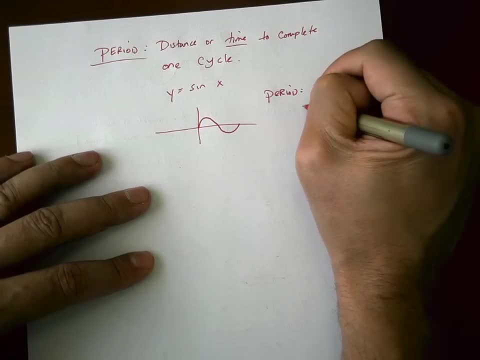 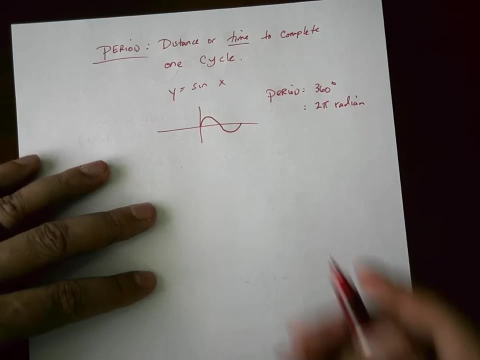 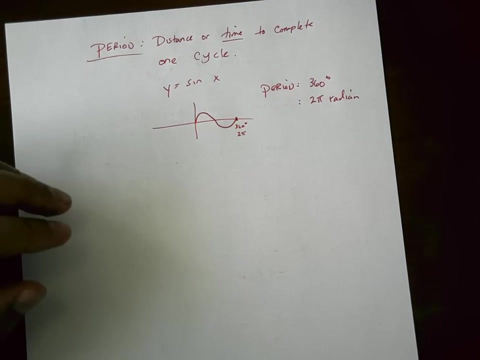 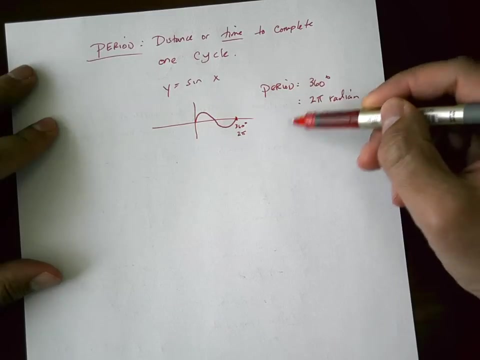 I could say it's 360 degrees. I could say it's 2 pi radian, That's how long it's taking to complete one cycle. So when you have a horizontal stretch or a horizontal compression, you're basically either making it longer to complete a cycle, more time. 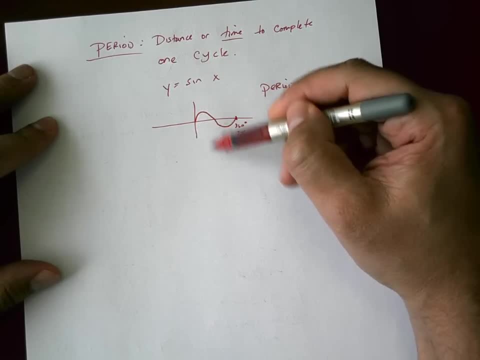 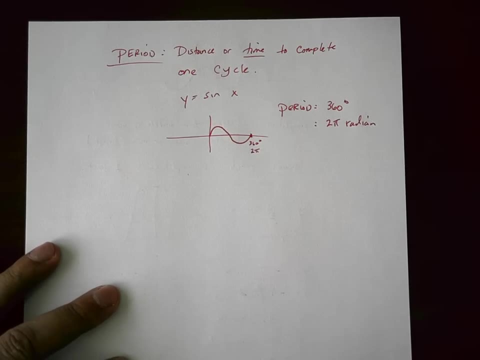 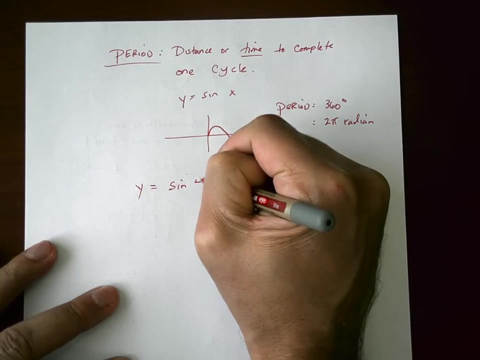 or you're making less time. You're making less time to complete a cycle because there are more cycles being completed in 360 degrees or 2 pi radian. So that's when we were talking in class today about. in class it was y equals the sine of 4x. 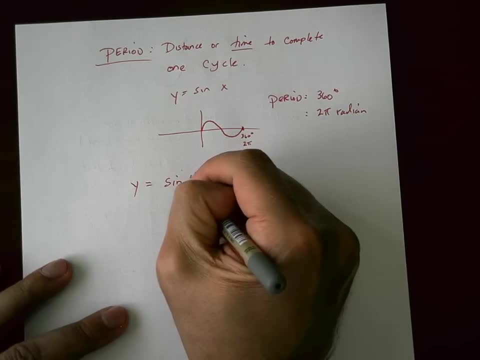 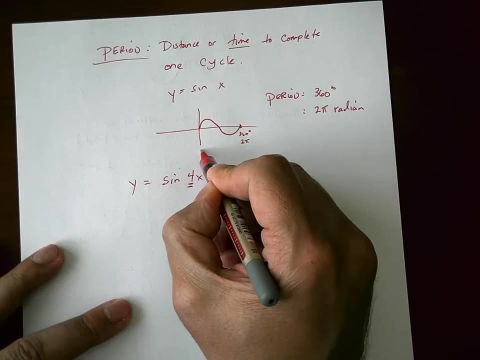 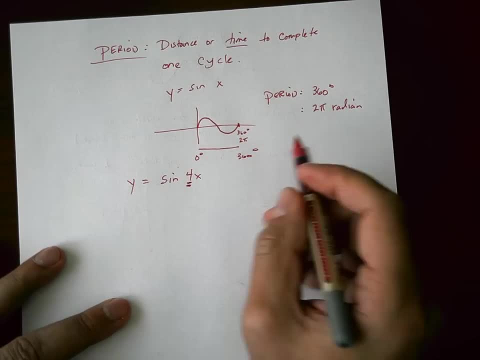 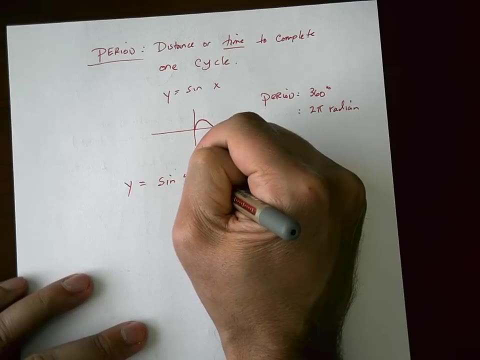 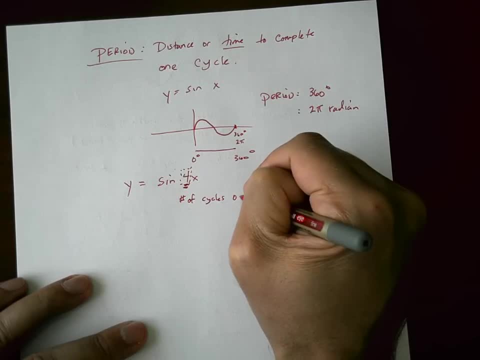 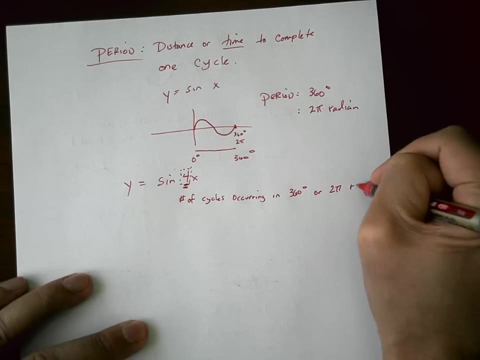 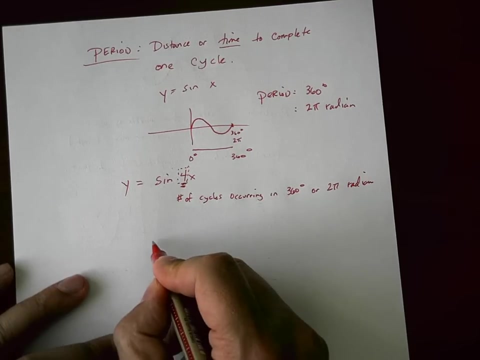 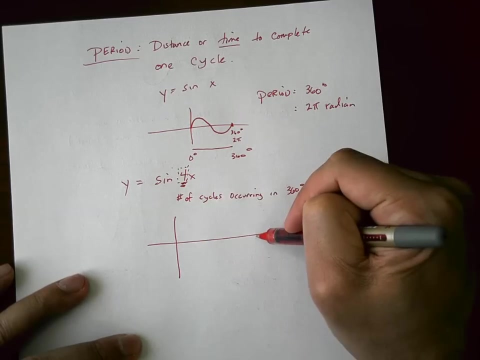 of cycles occurring in 360 degrees, or 2 pi radian Four cycles. So it took a while in class, but eventually I think we got to the point where, if this is at 0, and we claim this is 360 degrees, 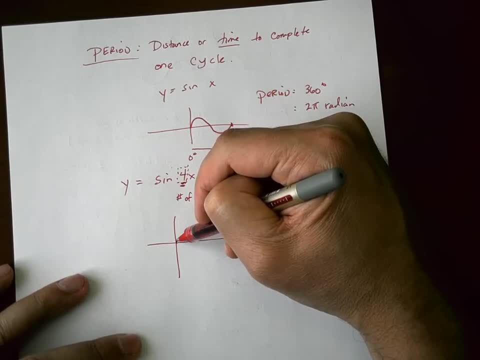 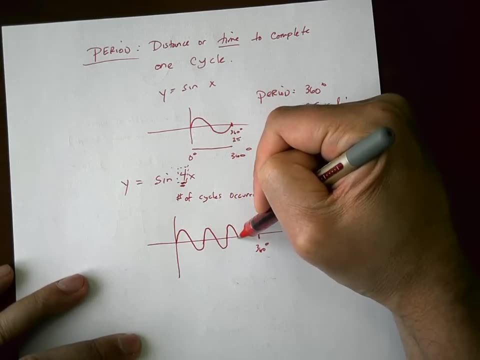 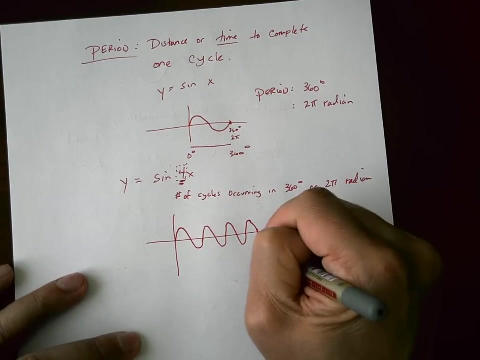 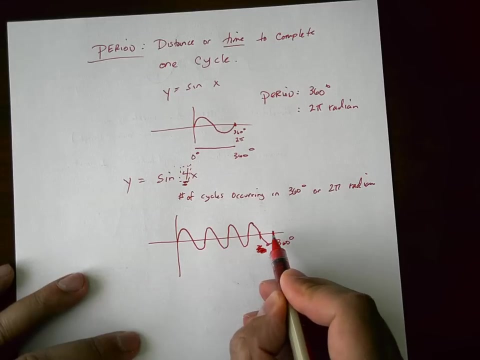 we say there's going to be four cycles- Now my spacing I don't know how good I'll do here- 1,, 2,, 3,, uh-oh, 4. 4.. So there's four cycles: 2,, 3,, 4, happening in 360 degrees. 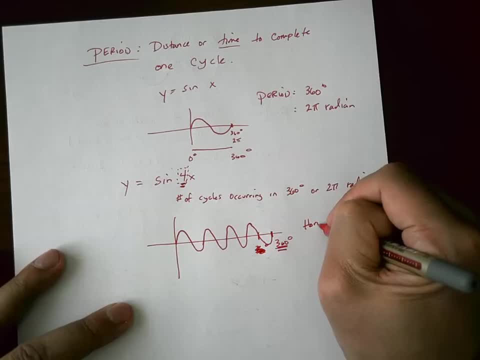 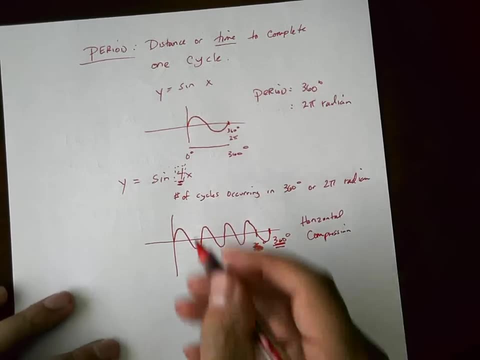 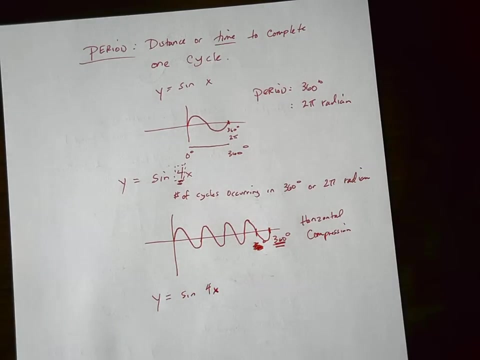 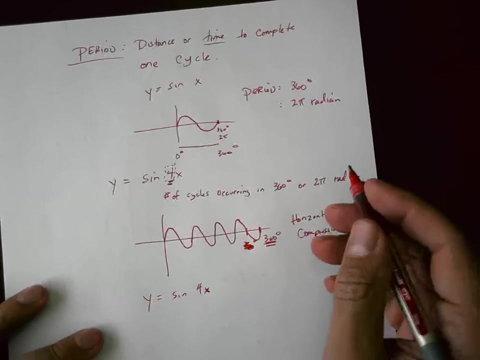 That is a horizontal compression. But the question becomes: what is the period of the function? Now, I wasn't calling it the period, but I was trying to get people to understand how long was it taking to complete one cycle? And it didn't come very easy for us to figure out. 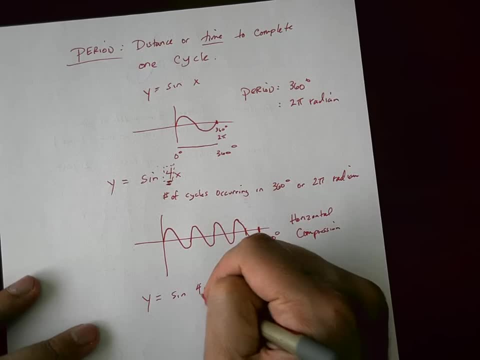 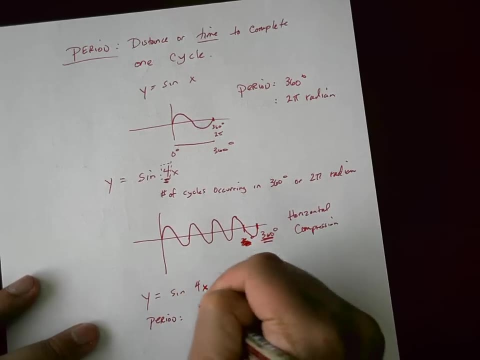 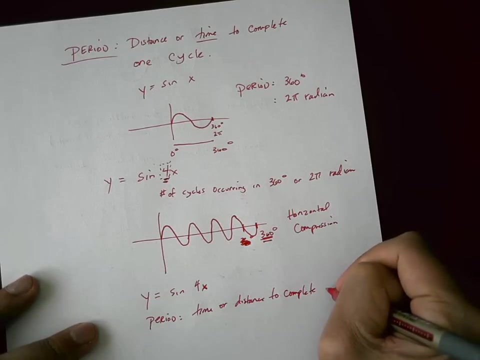 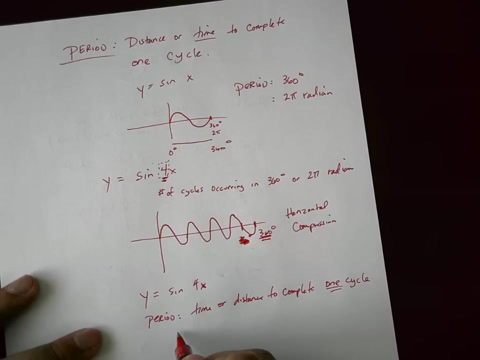 that if there are four cycles happening in 360 degrees- the period, the time or distance to complete one cycle, well, we'd have to take, in this case, 360 degrees, 360 degrees, and divide it by 4.. 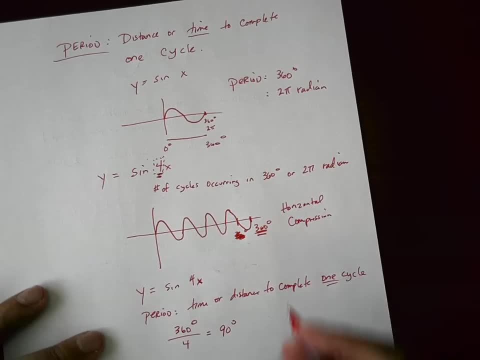 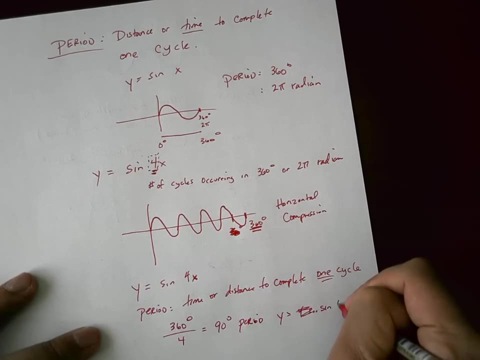 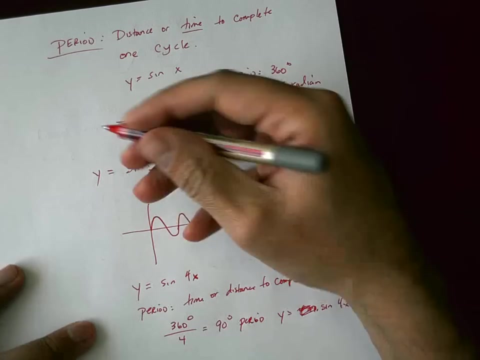 And you'd say: oh, 90 degrees is the period of y equals 4 times, or, excuse me, the sine of 4x. So what used to be happening on the parent in 360 degrees is now happening in just 90 degrees. 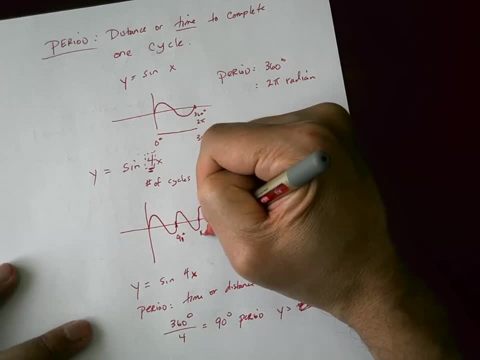 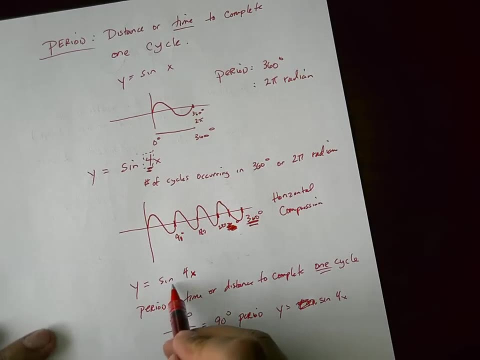 90 degrees, we complete a cycle. At 180,, we've completed a cycle. At 270,, we've completed 3.. And at 360, we've completed 4.. That's the sine of 4x. So in radian you wouldn't be taking 360 and dividing it by 4.. 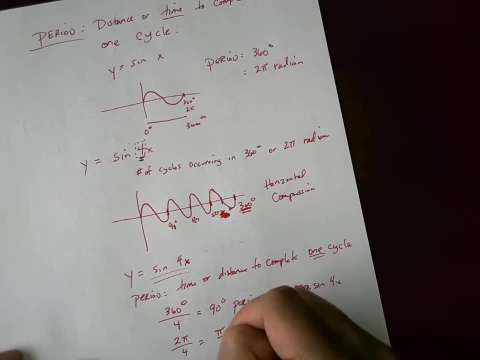 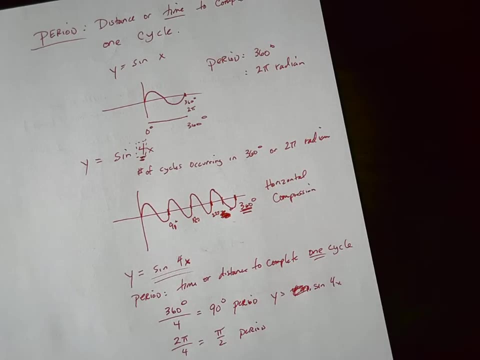 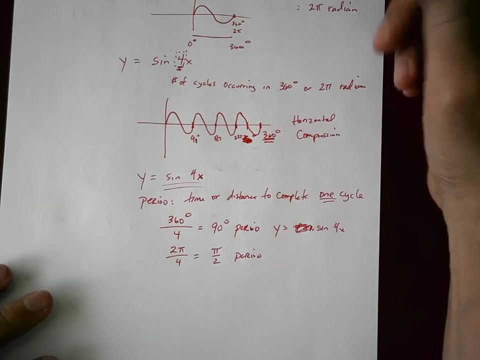 You'd be taking 2 pi and dividing it by 4 and saying pi over 2 is the period 90 degrees. So when they give you a function on the assignment, they're going to give you a function and they'll have some value that the input's getting multiplied by. 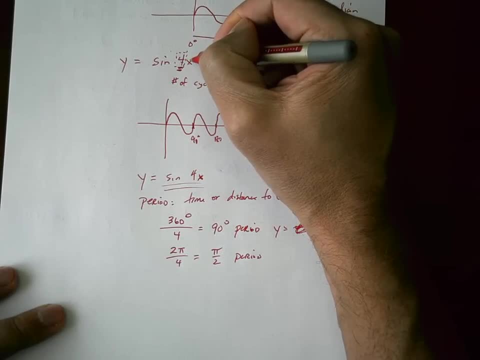 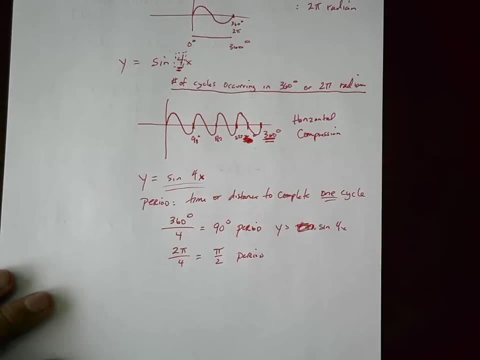 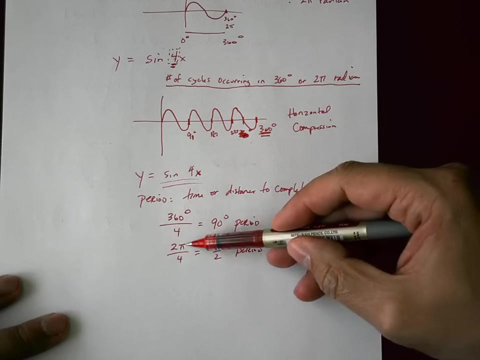 The value that the input is getting multiplied by is not the period. It's the number of cycles occurring in 360 degrees or 2 pi radian. To find the period, you have to take that 360 degrees or take that 2 pi radian. 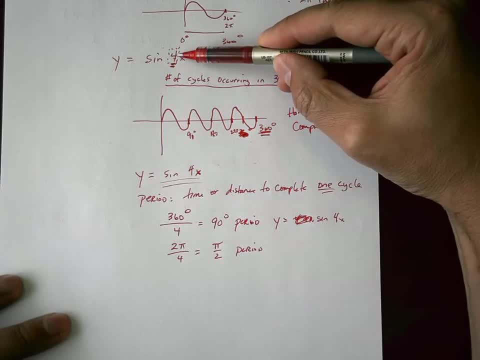 It's always going to be 2 pi radian. You have to divide it by how many cycles are happening in 2 pi to figure out how many cycles are happening in 2 pi And you have to figure out what the period is. 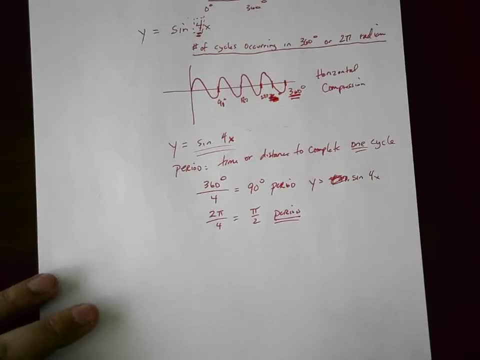 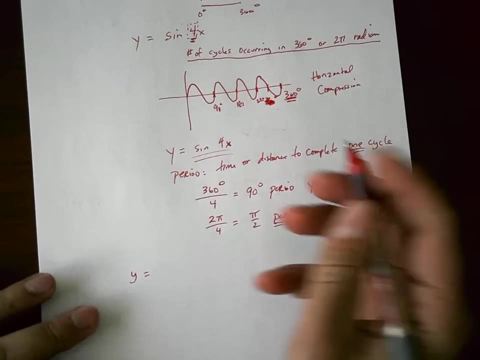 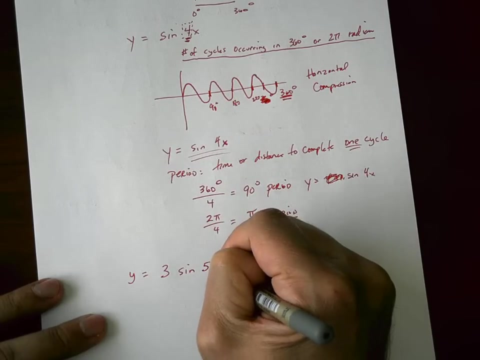 So they will give you on the assignment, they'll give you functions and it'll say, like y equals 3 times the sine of 5x, And they'll ask for the amplitude. You'll say, well, the amplitude. 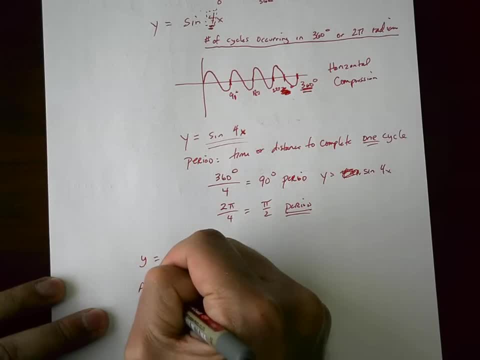 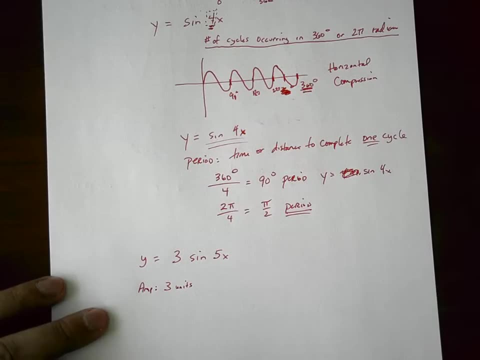 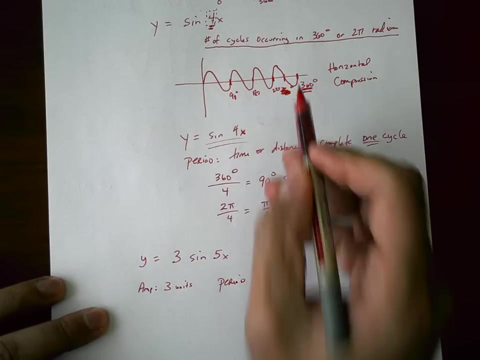 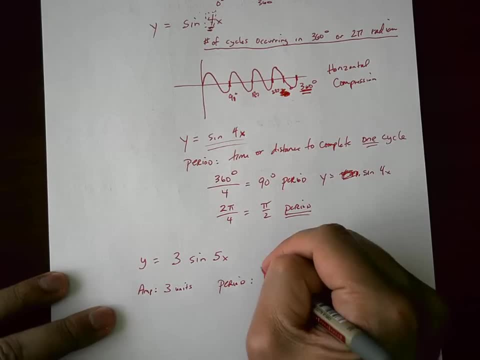 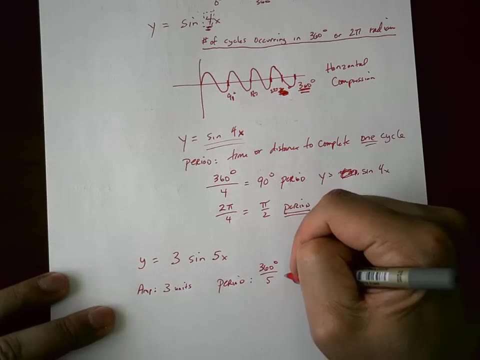 Now they're not going to deal with degrees. Yes, you could say 360 degrees divided by 5, which does that even work out nice 74, right? 75, 35, 10,, 72. That'd be 72 degrees. 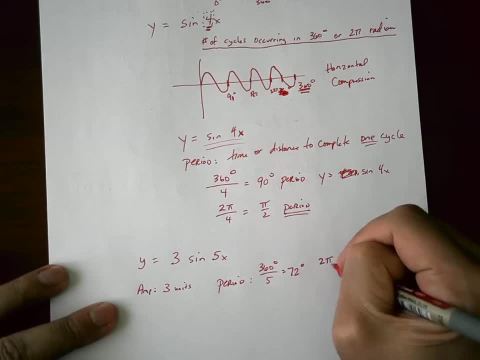 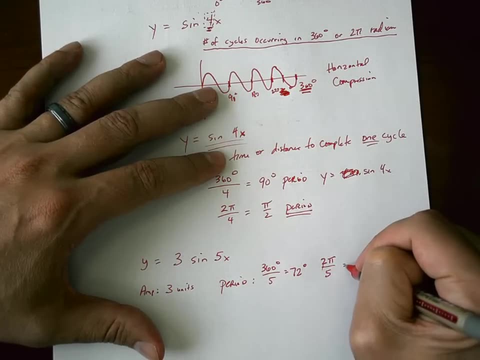 But when you look in the back they're going to have taken 2 pi and dividing it by 5, and that doesn't really simplify. so they'll say 2 pi divided by 5 is the period. 2 pi over 5 in degrees must be 72 degrees. 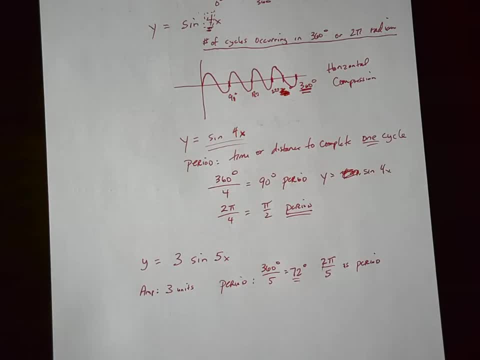 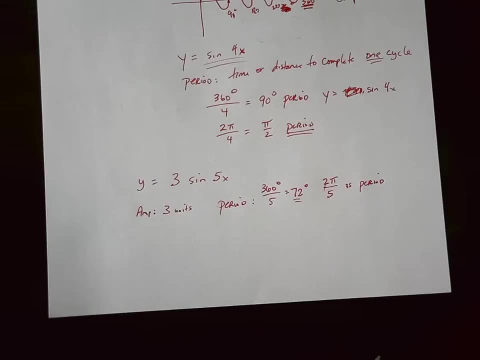 You convert 2 pi over 5 to degrees, you get 72 degrees. If The value that the input's getting multiplied is in terms of pi, Boy, students get really flustered. They get really flustered like: 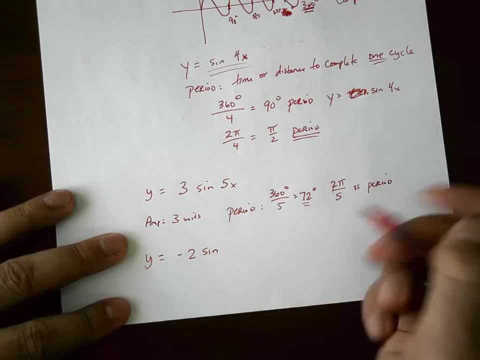 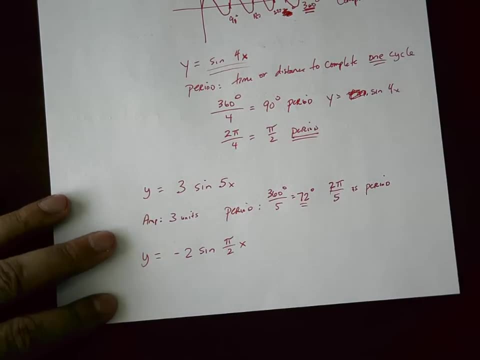 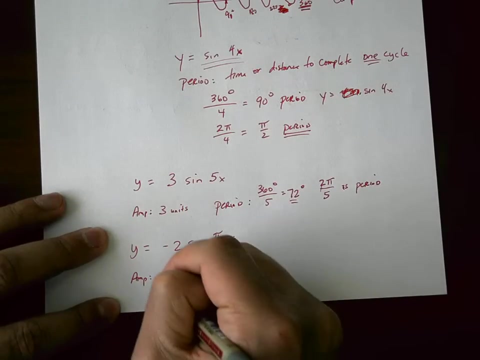 when it'll say negative 2 times the sine of and they'll put pi over 2x instead of saying like 5x. Say what's the amplitude? The amplitude is 2, not negative 2.. There's just a. 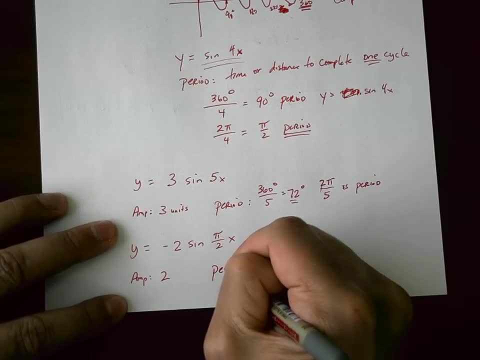 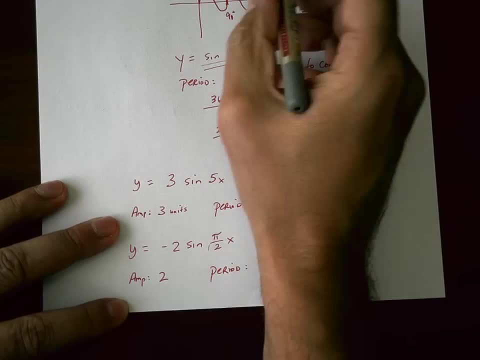 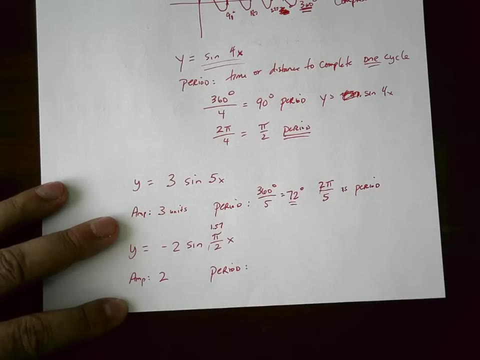 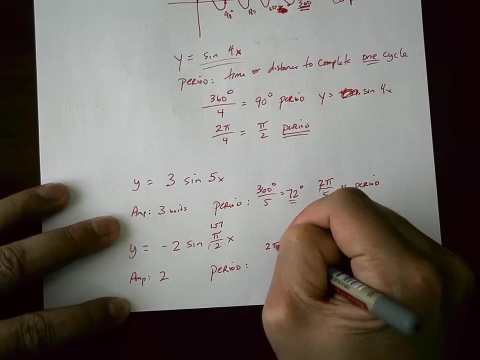 If you say, oh, to get the period, I have to see this is 5 cycles occurring in 360. Well, this is about 1.57 cycles occurring in 360.. So you need to take 2 pi, which is the normal period of the parent. 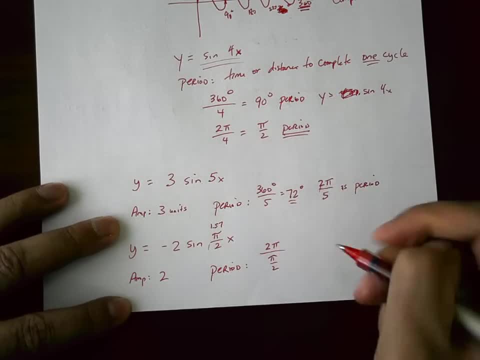 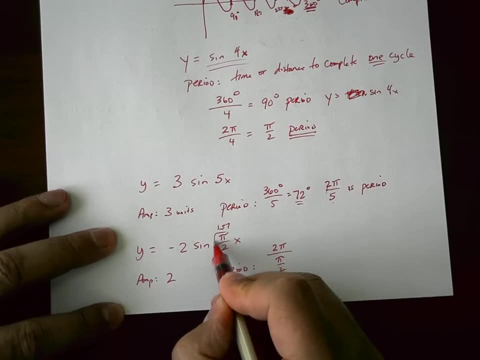 and you have to divide it, and you have to divide it by pi over 2.. It's no different than taking 2 pi and dividing it by 5, because there was a 5 there. Now we're taking 2 pi and dividing it by pi over 2.. 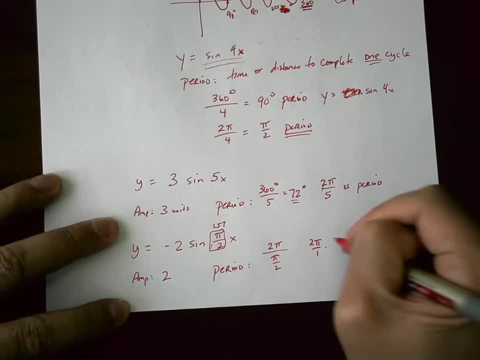 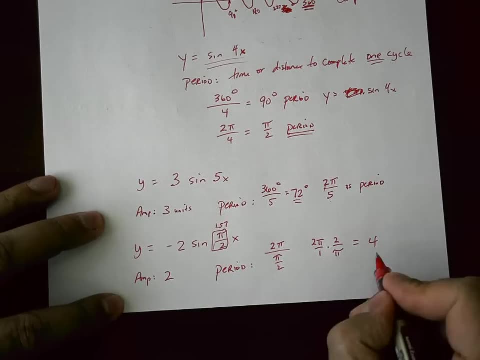 What happens? That means 2 pi over 1, multiplied by the reciprocal 2 over pi, and you just get 4.. And students don't know what to do with the 4. They're like 4? The period is 4?. 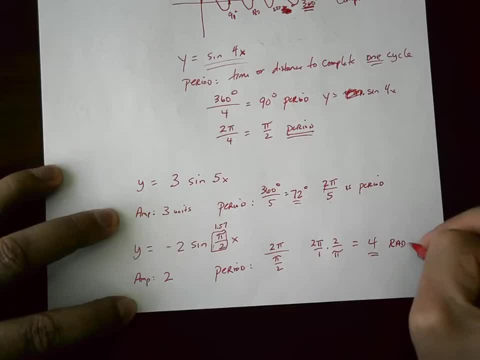 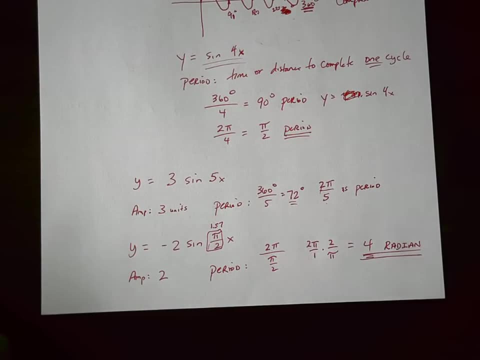 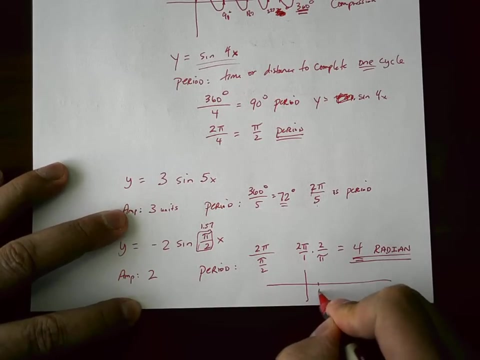 4. what 4 radian? So the answer is that 1 cycle is being completed in 4 radian. So, graphically, if your inputs were in radian and you say here's 1,, here's 2,, here's 3,, here's 4,. 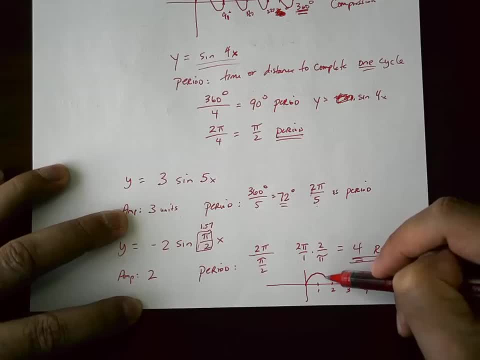 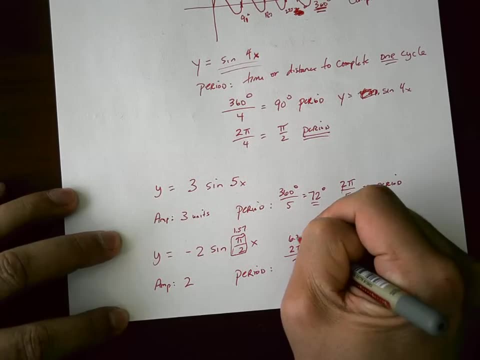 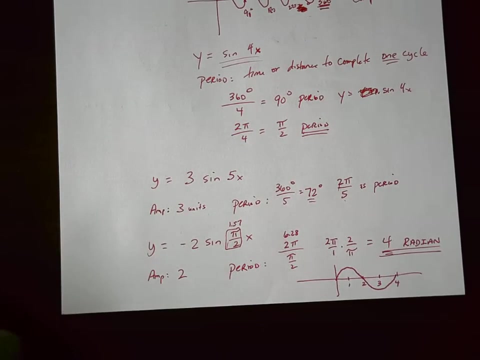 you're completing a cycle in 4 radian instead of 6.28.. It's not taking 6.28 radian to complete a cycle. It's taking only 4 radian to complete a cycle. It's a horizontal compression. 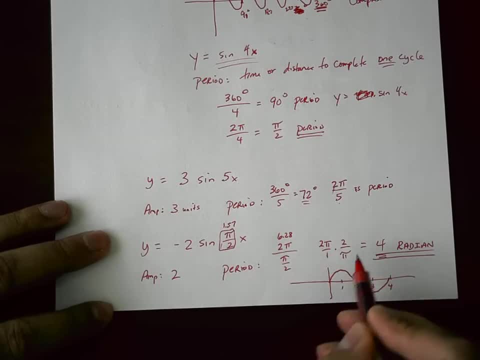 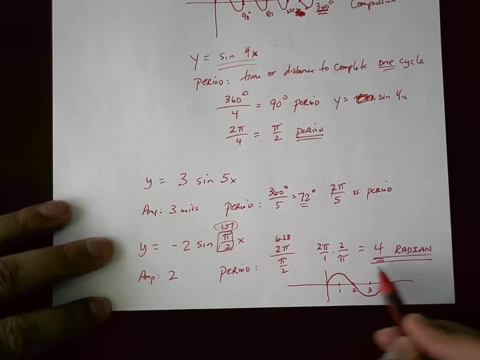 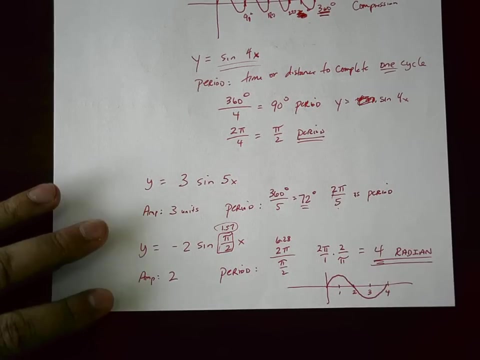 Instead of only completing 1 cycle in 6.28,, we're completing 1.57 cycles in 6.28.. So the period is 4 radian Up here, when there was a 5 here and you say 2 pi divided by 5,.